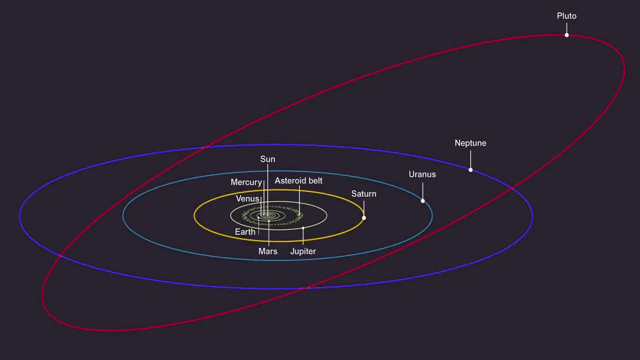 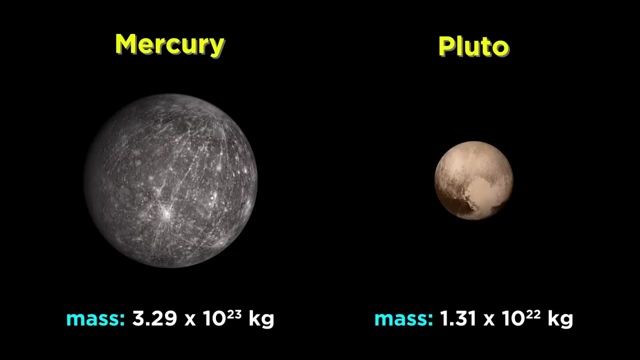 Far from any anti-canine sentiment, this decision had a firm logical basis. Besides Pluto's tilted and eccentric orbit, Pluto is much, much smaller than any of the planets, with a mass less than one tenth of the smallest planet, Mercury. Pluto is smaller even than our own moon, although it actually has several moons of its own. 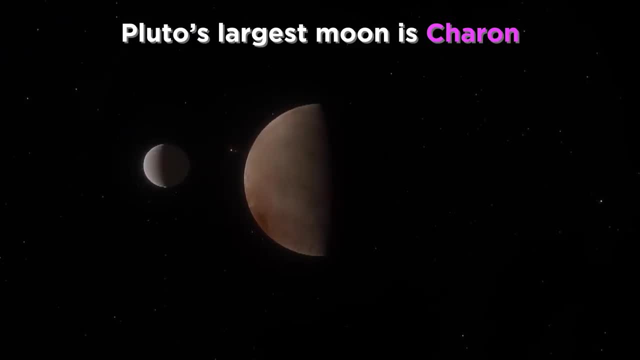 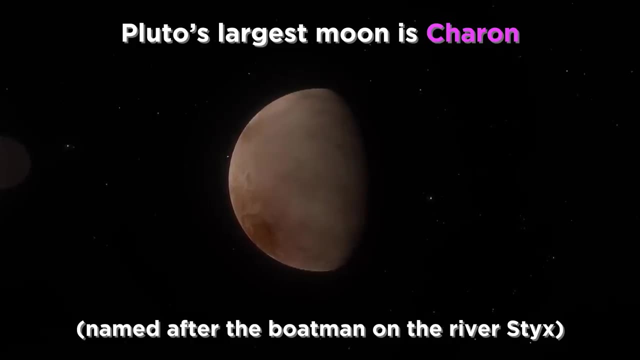 Pluto is smaller even than our own moon, although it actually has several moons of its own. The largest of these, Charon, is named after the boatman who ferries dead souls across the river Styx into the underworld. But more important than all this, orbiting at a comparable distance to Pluto are many. 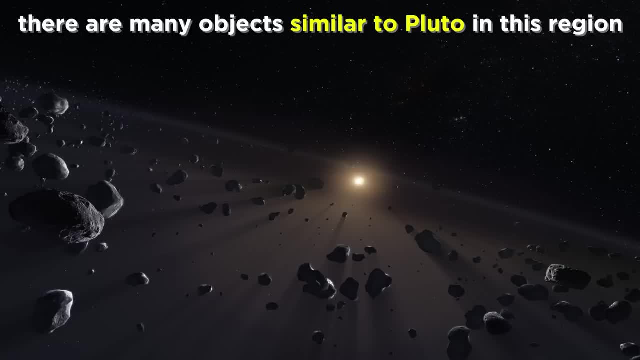 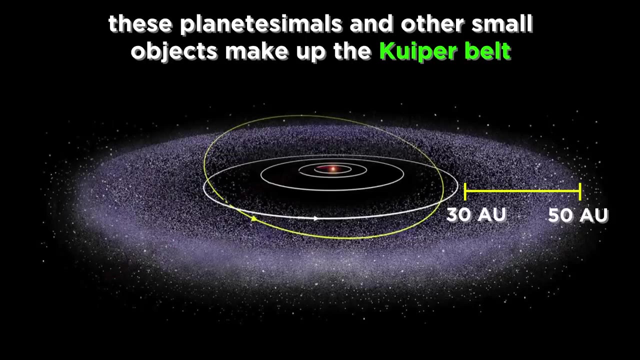 other objects that are quite similar, some of which rival Pluto in size. What are these things? They are planetesimals and other small objects remnants from the birth of the solar system, and they form a region called the Kuiper belt, extending from around thirty to fifty astronomical. 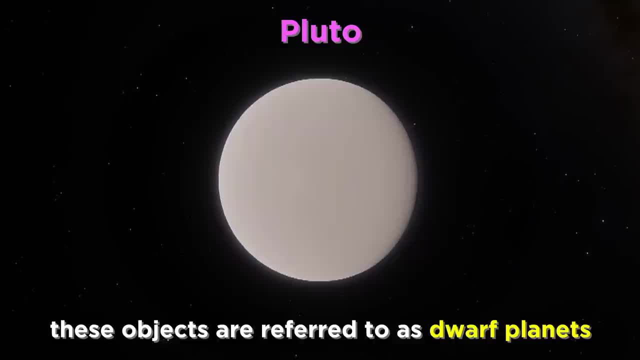 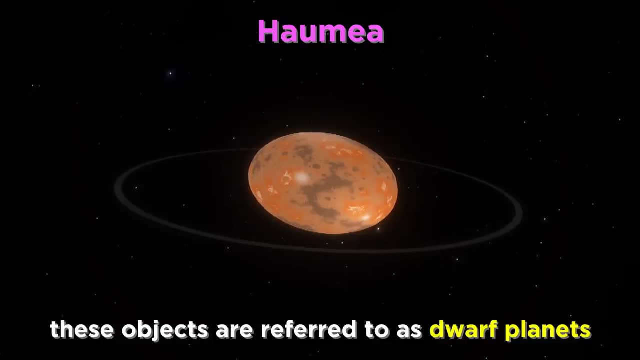 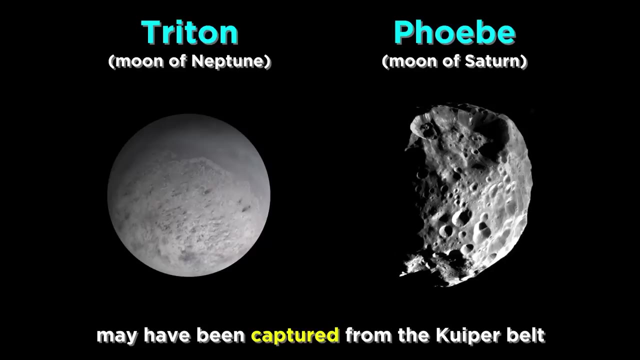 units from the sun. Pluto is one of three dwarf planets in this region, and it is thought that several moons in the solar system also originated from this region and were captured by planets like Triton around Neptune and Phoebe around Saturn. 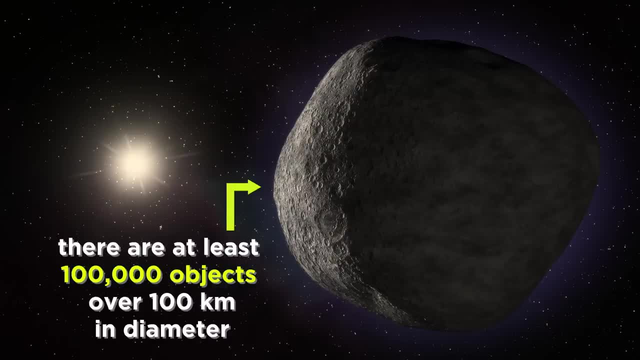 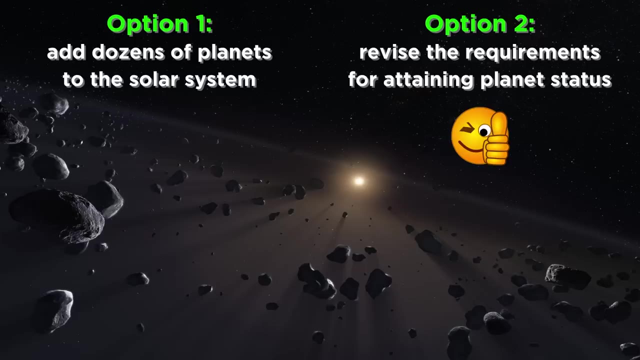 Beyond these dwarf planets, there are at least a hundred thousand smaller objects that are over a hundred kilometers in diameter, sharing the same composition as Pluto. This understanding required that, rather than adding dozens of new planets to the solar system, we should revise the definition of the word planet, and we decided that in order 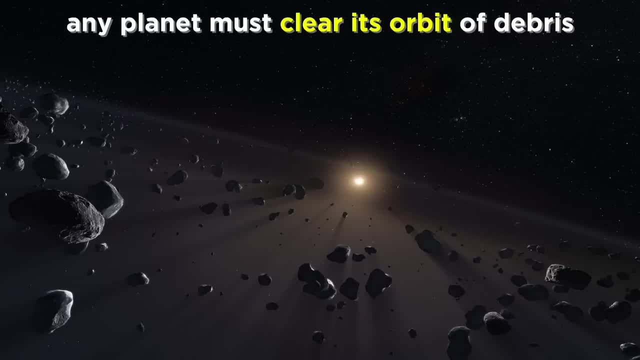 to qualify as a planet, an object must clear the region near its orbit of other debris. As Pluto is surrounded by planetesimals, some of which are similar in size and also have known satellites, it was determined that Pluto should not qualify as a planet. but 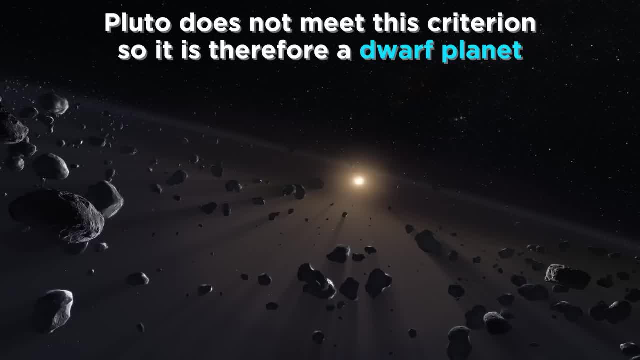 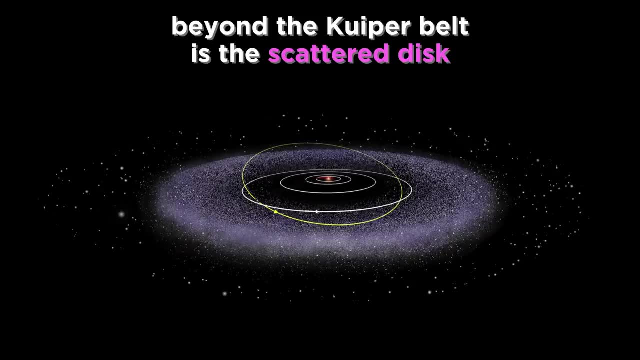 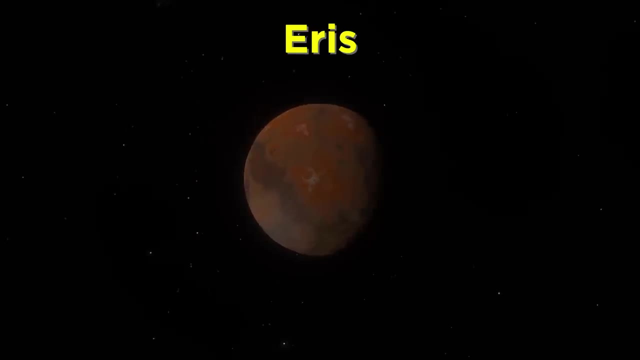 will rather be referred to as a dwarf planet, as will several other large objects in the Kuiper belt. Beyond the Kuiper belt is a region called the scattered disk, extending to one hundred astronomical units from the sun. This region contains another dwarf planet called Eris, which is slightly more massive. 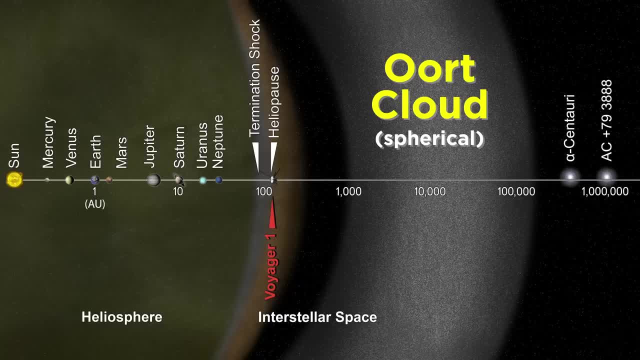 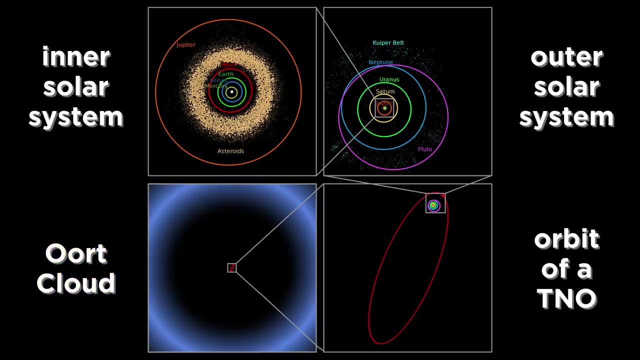 than Pluto. Much farther still is the theoretical Oort cloud, a spherical region tens of thousands of astronomical units from the sun, And there you have the outer regions of the solar system, which probably make it quite a bit larger than you may have thought. 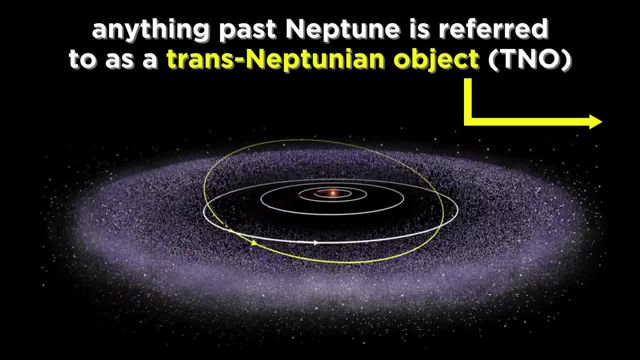 Starting with the Kuiper belt and moving outwards. all of these regions contain what we refer to as trans-Neptunian objects, which just means anything beyond the Oort, And it is these outermost regions that comets come from. 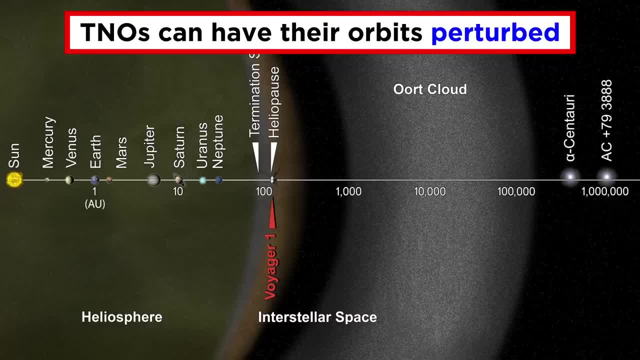 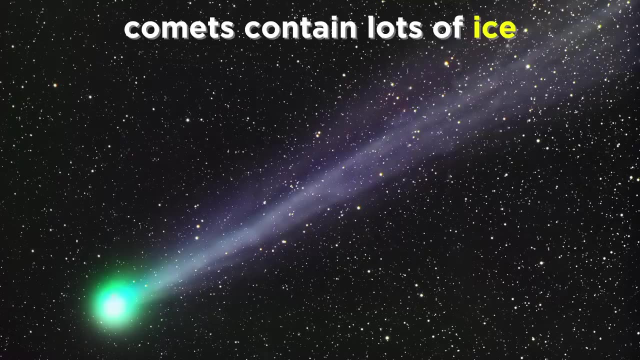 Objects orbiting as far as the Oort cloud can still have their orbits perturbed by the gravitational influence of the gas giants or even by other stars in the Milky Way that are passing by and are then sent towards the sun in highly elliptical orbits. 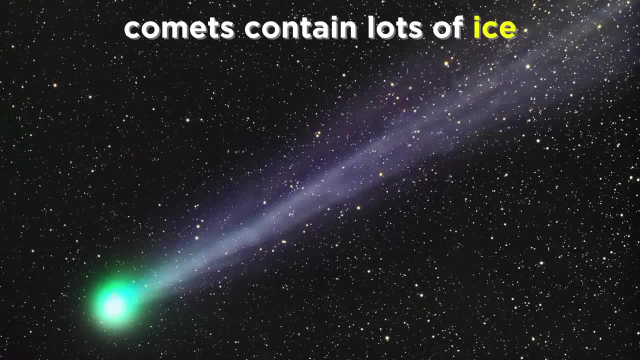 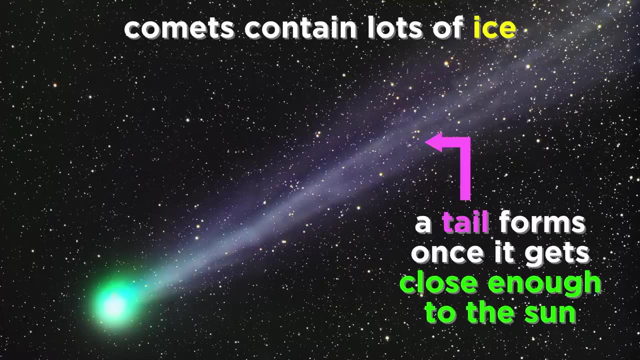 As they originate far away from the sun, they are very icy, But as they get closer to the sun they heat up, which melts the ice. Once they are about as close as Jupiter, this vaporized water, along with the gas and dust, 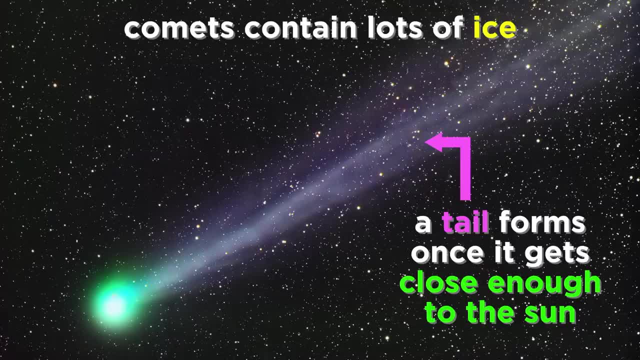 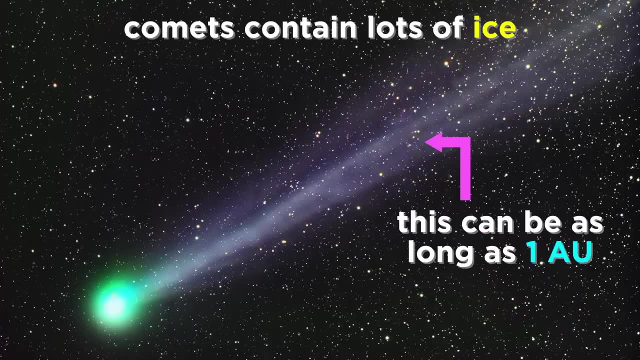 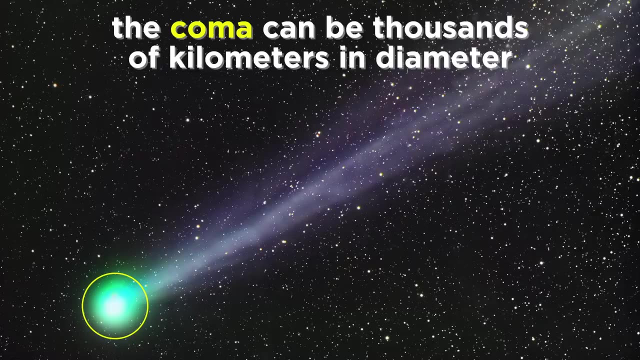 trapped within, gets pushed out by radiation pressure from the sun and becomes the tail of the comet, which can grow as long as an entire astronomical unit held in place by the solar wind. This tail emerges from a cloud of gas called the coma, which is thousands of comets that 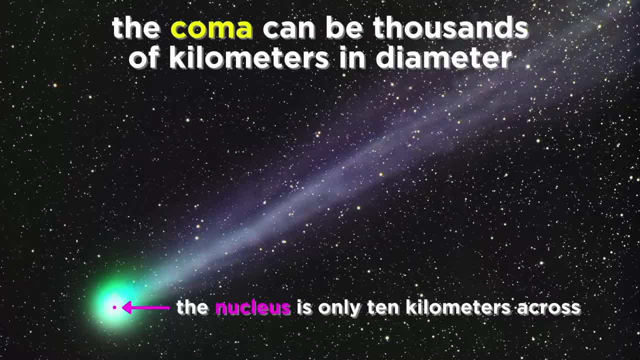 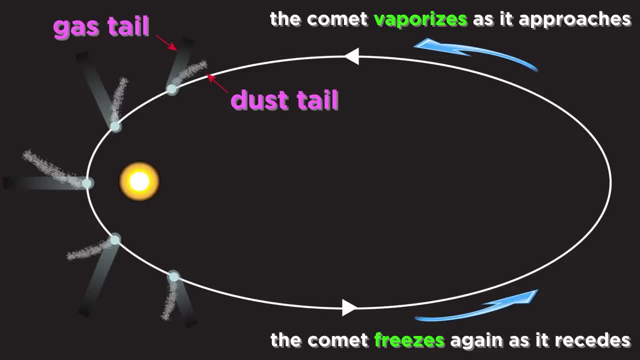 are thousands of kilometers across, even though the nucleus of the comet itself is very small, maybe around ten kilometers across a block of ice and gas that melts as it approaches the sun and then freezes again on its way back to the outer solar system, only to return. 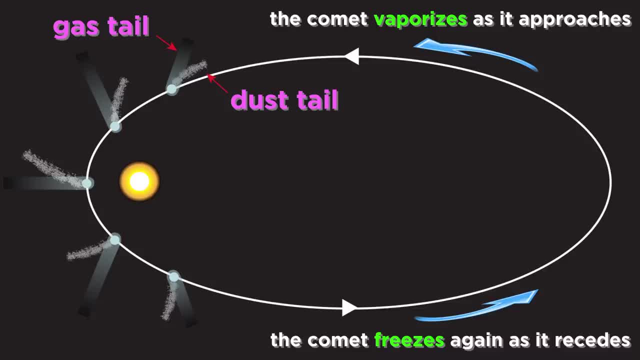 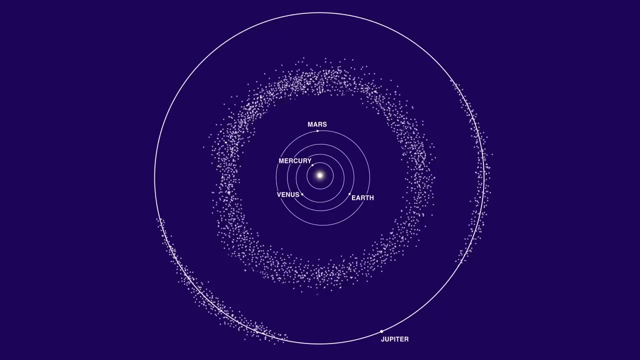 many years later, often millions of years later. But it's not just the outermost region of the solar system that contains small objects In between the orbits of Mars and Jupiter. there are also small objects In between the orbits of Mars and Jupiter. there are small objects. 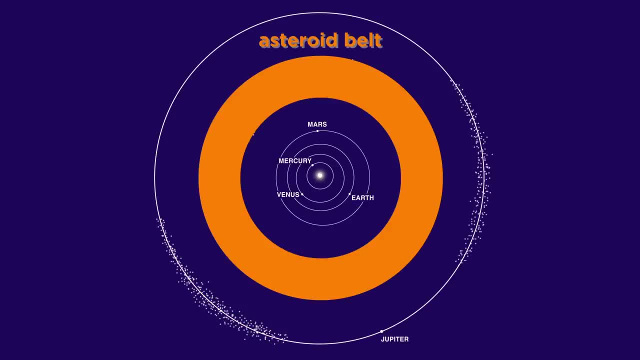 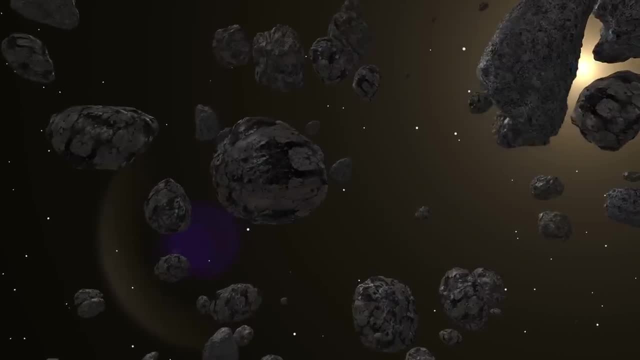 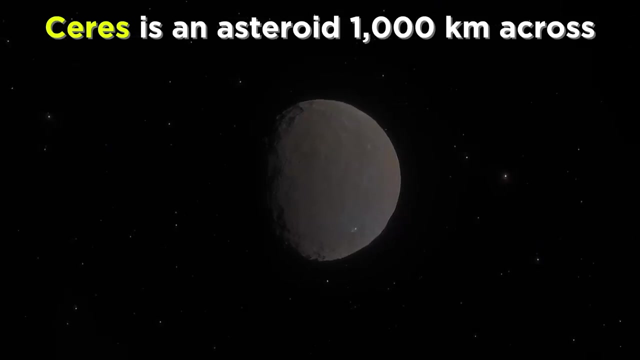 In between the orbits of Mars and Jupiter, there is the asteroid belt. This is comprised of thousands of small rocks, just like the kind that came together to form planetesimals in the early solar system. They range in size from around a thousand kilometers across, at their largest like an. 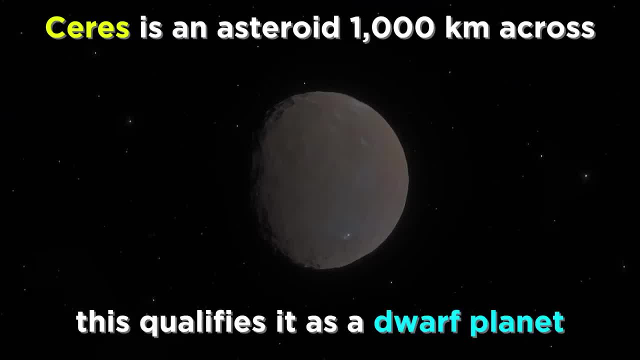 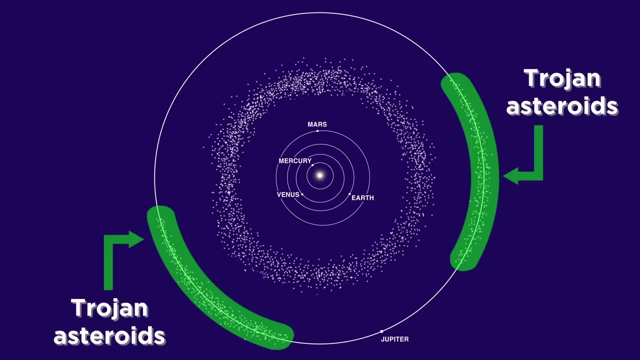 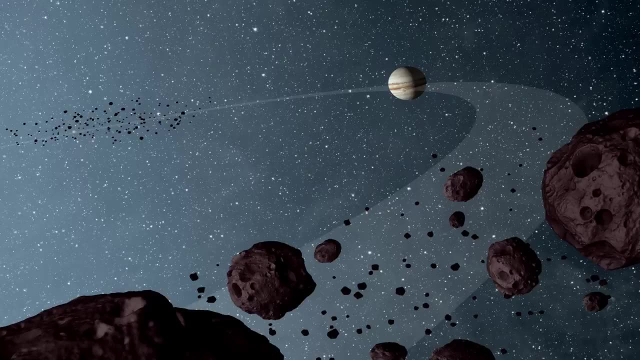 asteroid named Ceres, which is large enough to qualify as a dwarf planet, down to very small rocks just a few meters across. There are also two patterns. There are two patches of asteroids, called Trojan asteroids, that lie directly on Jupiter's orbit and orbit with the same period as Jupiter. 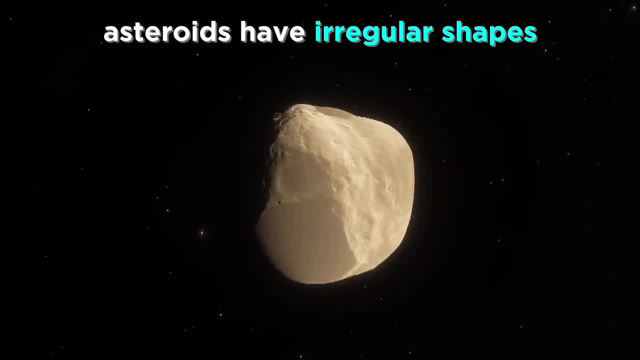 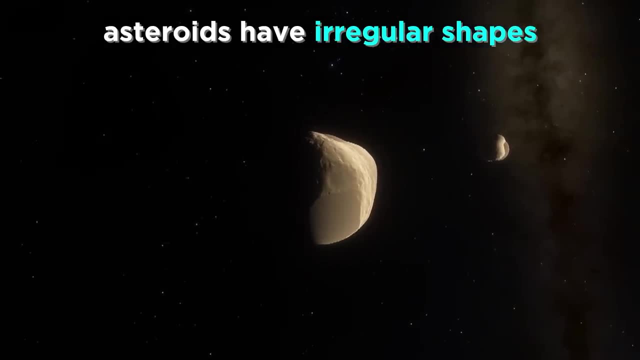 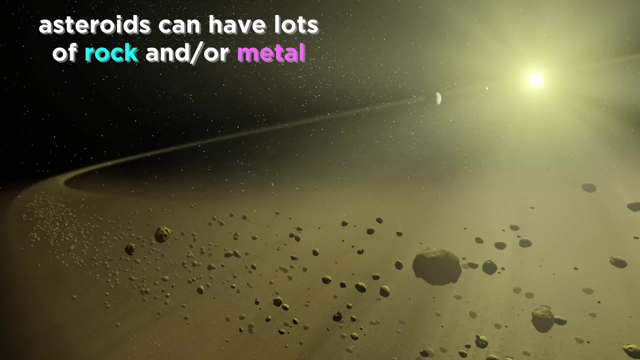 Most asteroids are too small to be crushed into spheres by their own gravity, so they have irregular shapes, and frequent collisions blast away chunks to form new irregular shapes. Some asteroids are very rocky, some have lots of metal and some have both. So why didn't these rocks gather to form a planet, like they did for the other planets? 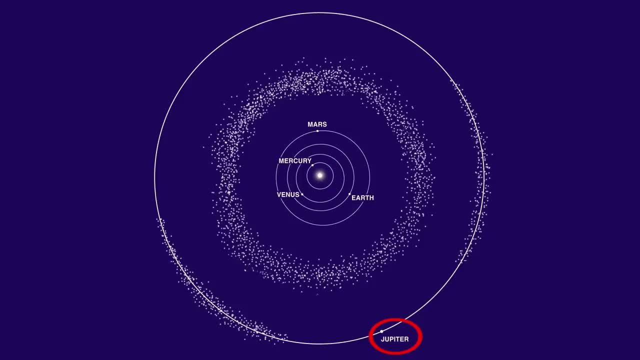 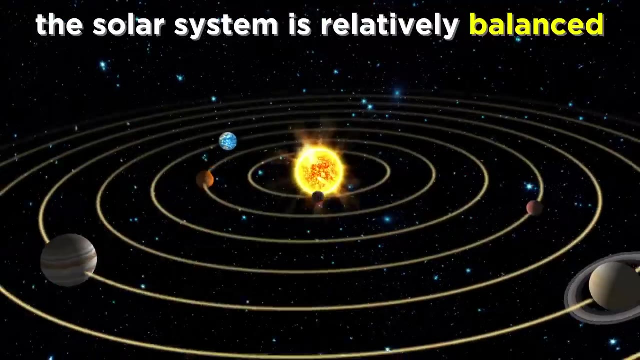 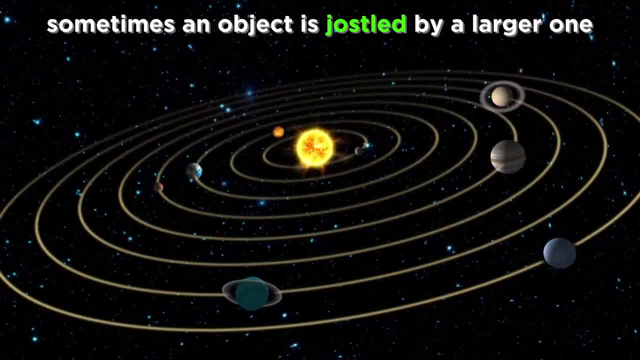 Planets continue in their orbits, which is why they have such a strong gravitational pull. Planets continue in their orbits, which is why they have such a strong gravitational pull, But sometimes small objects can be jostled by the gravitational influence of larger. 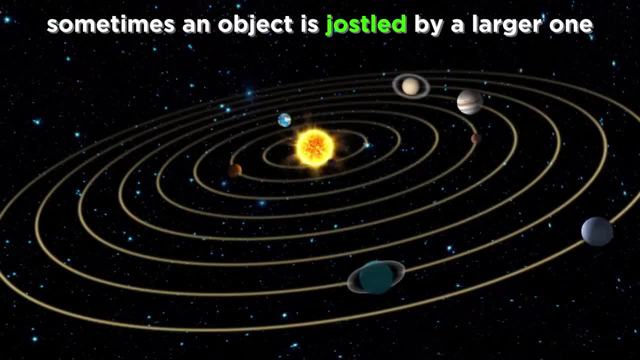 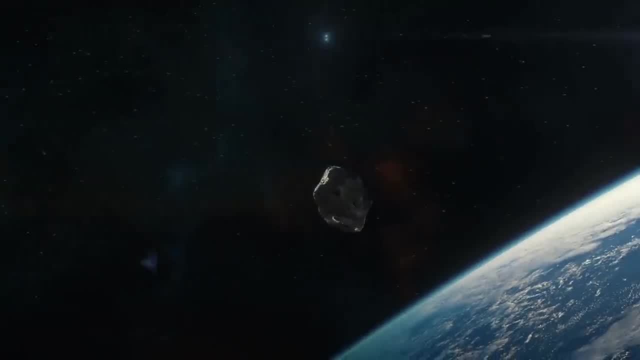 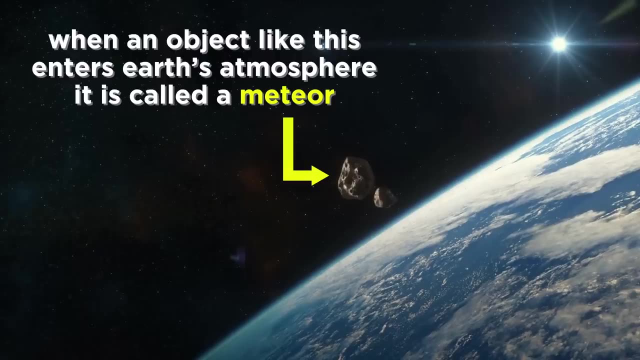 objects and are sent on rogue trajectories. Once in a while such a trajectory could result in a collision with a planet, even Earth. When such an object enters Earth's atmosphere, we call it a meteor. So really a meteor is just any rocky object, like an asteroid, that can hit an object that 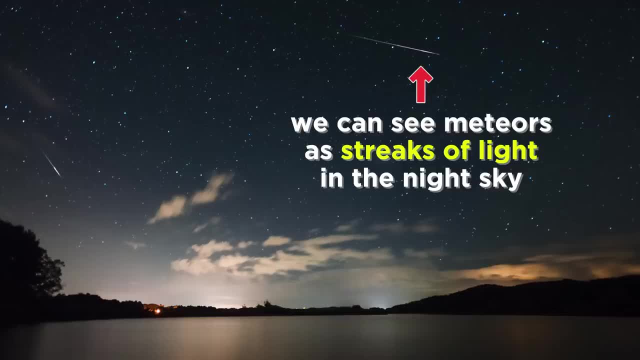 like an asteroid that makes it to Earth. These are visible in the night sky as brief streaks of light and they are often referred to as shooting stars. This is because they are so small relative to the stars that they resemble stars in the 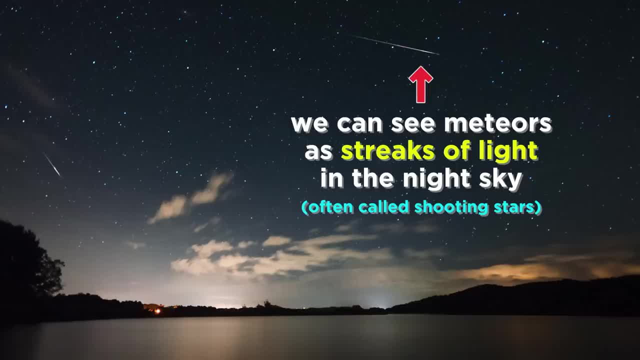 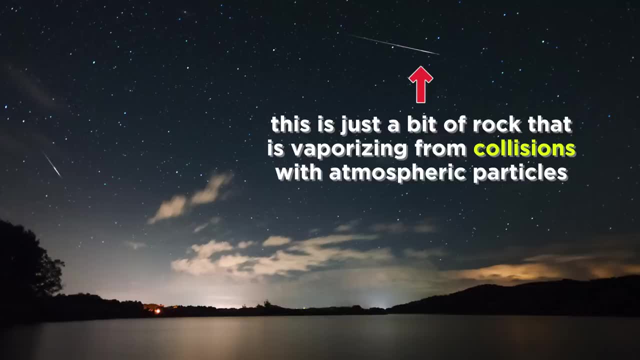 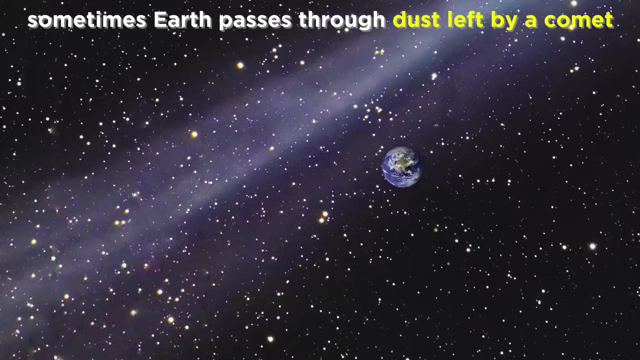 night sky, even though they are within Earth's atmosphere. But once again they are just bits of rock that heat up from all the friction due to colliding with particles in the air, which leaves behind a trail of vaporized material. Sometimes Earth passes through a trail of dust that was left by a comet approaching. 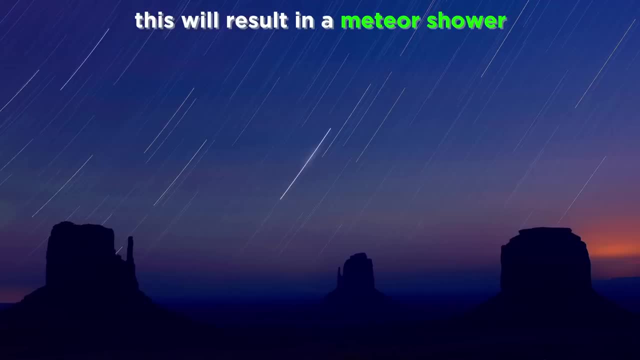 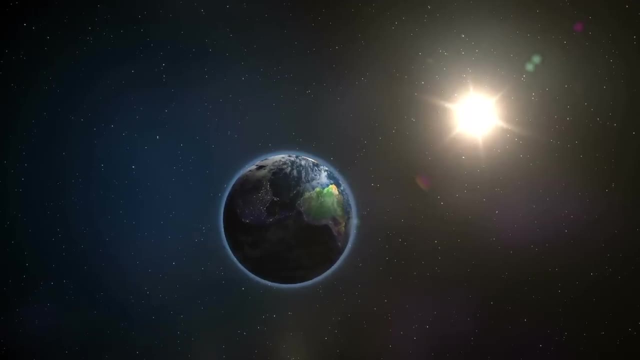 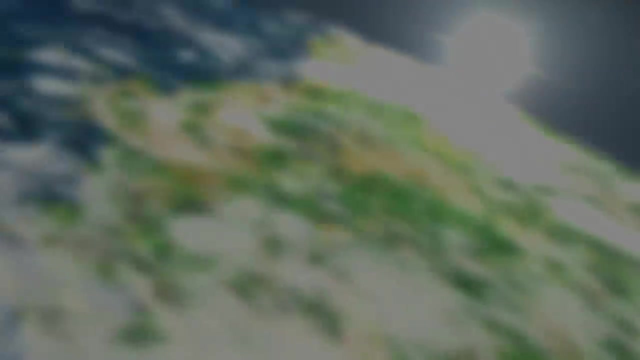 the sun, and in such an instance, many particles will rain down in a short period of time. This is called a meteor shower, But even under normal circumstances, Earth is constantly being bombarded by these types of objects, Thousands of them every minute. 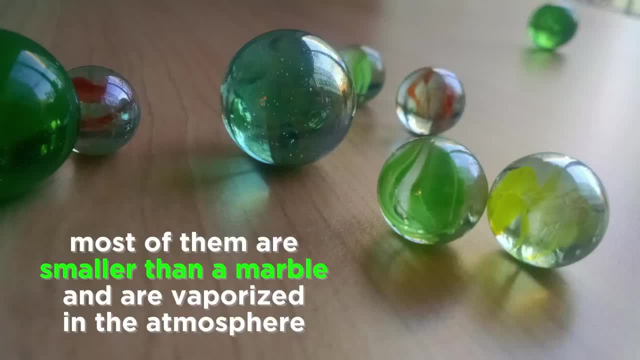 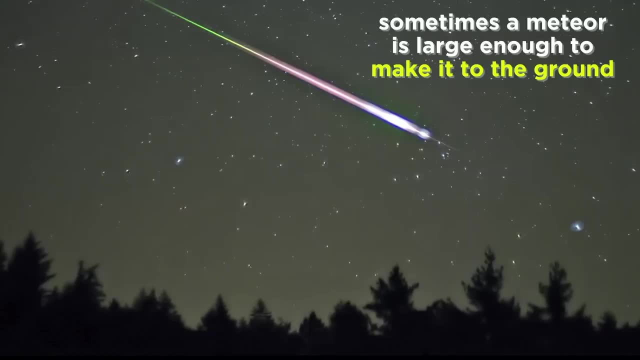 But most of them are very small, smaller than a marble, and are usually completely vaporized in the atmosphere. But if they are large enough, some remnant of the meteor will make it to the ground and once a meteor touches the ground it's called a meteorite. 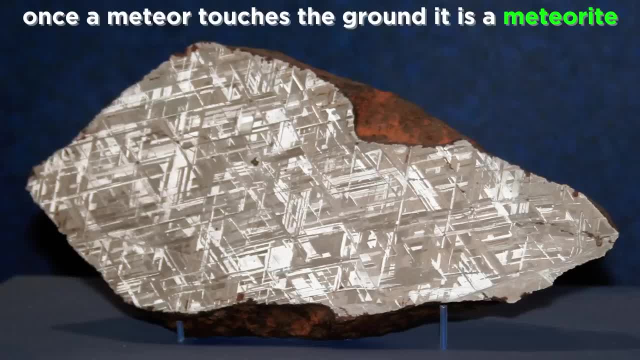 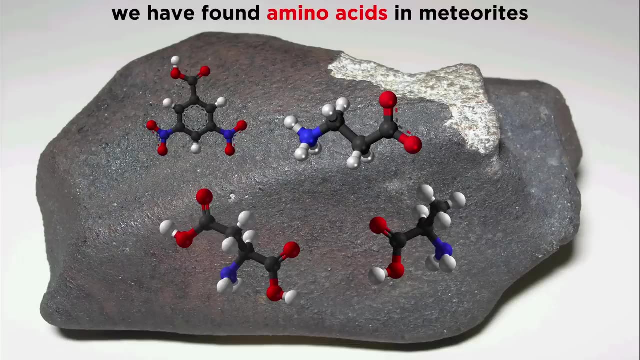 These objects are quite valuable for studying the early solar system because they are remnants from that time, and analyzing the radioactivity of these objects is one way we can determine the age of the solar system. We have even found amino acids inside meteorites, which means that the basic building blocks 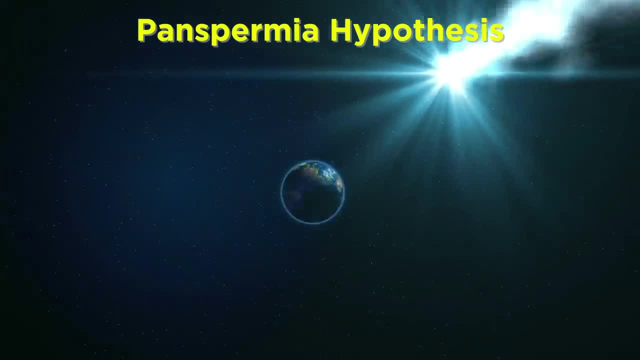 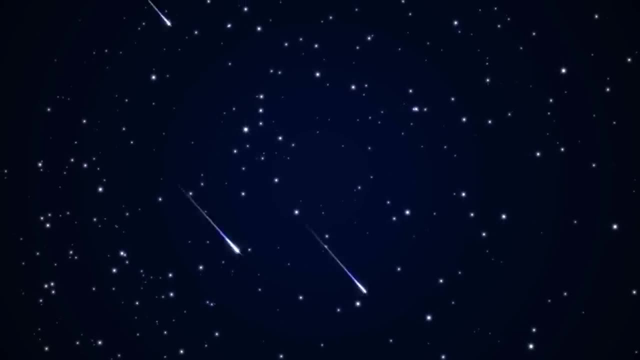 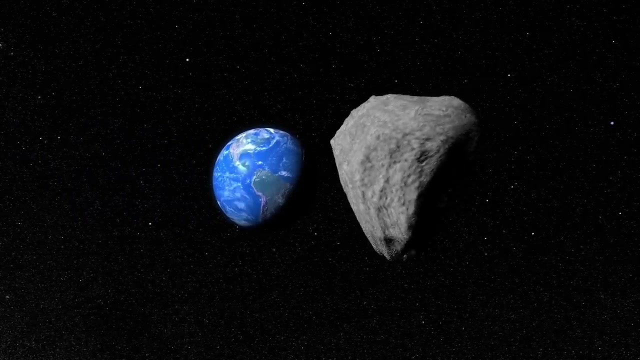 for life might have come from space, which is the basis for the panspermia hypothesis. It's not all laser shows and space parties with meteors, though. Every few thousand years, a meteor that is ten to a hundred meters across will collide. with the Earth. When meteors are this large, they release an enormous amount of radiation. This is called a meteor shower. This amount of energy on impact- A meteor the size of a house- would yield an impact with the same explosive power as a. 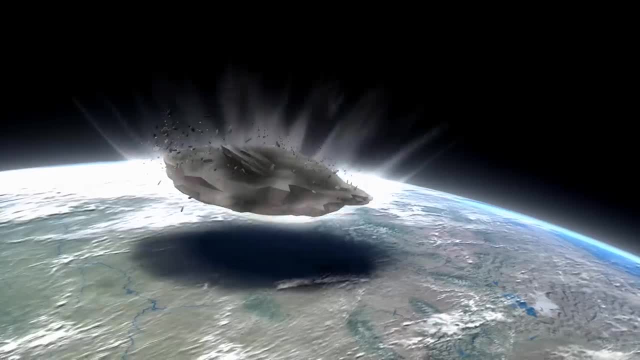 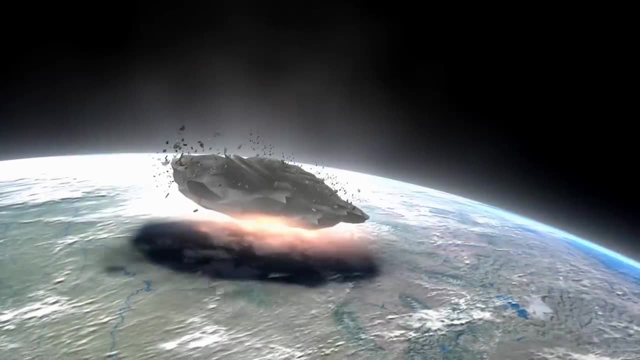 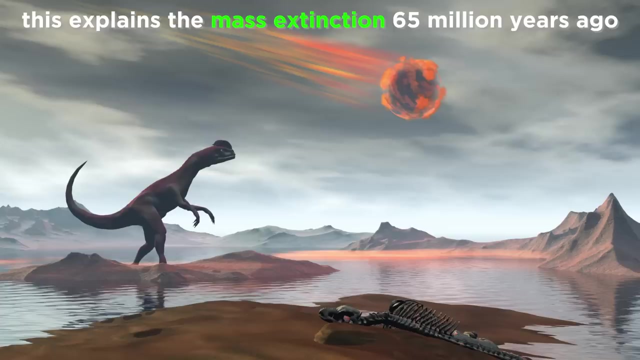 thermonuclear bomb. There is strong evidence of meteors much larger than this colliding with the Earth in the past, and we believe that such a catastrophic event, involving an asteroid ten kilometers across, is responsible for the mass extinction visible in the fossil record: 65 million years. 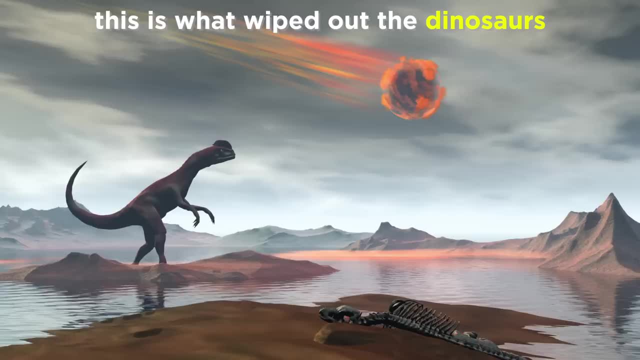 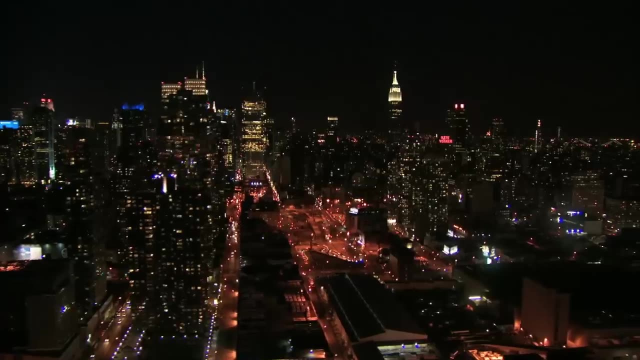 ago, resulting in the end of the age of the solar system, The age of dinosaurs and the rise of the mammals. Luckily, no event quite so jarring has occurred since then, or us mammals probably wouldn't be here to learn about it. so let's move forward and learn about some of the things.